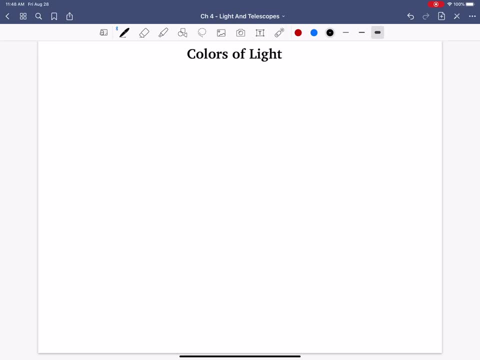 Okay. so anytime we talk about light, anytime, say astronomers measure light, there has to be a source of that light. So our go-to source is a light bulb, at least to explain this concept. So let's draw a stereotypical light bulb right, an incandescent light bulb to be exact. 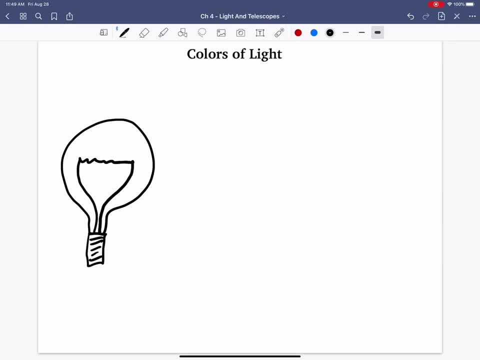 So incandescent light bulbs have a glass bulb that surrounds a very thin metal filament strung across two holders right. That's a very, very thin light bulb that surrounds a very thin metal filament strung across two holders right. delicate piece of metal And electricity is fed in one end passes across that thin metal filament. 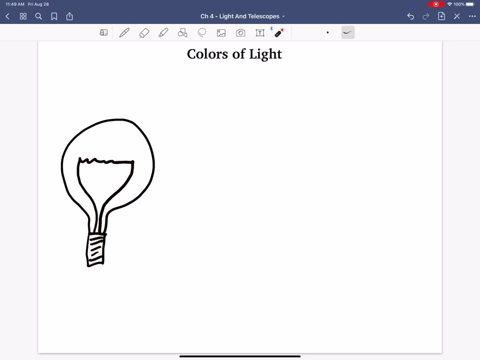 and out the other side right. That completes the electric circuit. And what happens as the electricity flows across the metal is that it heats up that metal to thousands of degrees right, Which is the temperature of some stars. So that's incredibly hot. 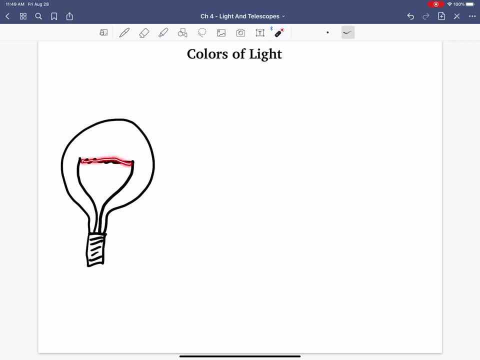 And that effect is manifested in the form of light. right, That's how these light bulbs will produce light. They glow, right. Specifically, the filaments glow And the type of light that we see. to our eyes it appears a pale yellow, right, That's because our eyes are most sensitive to. 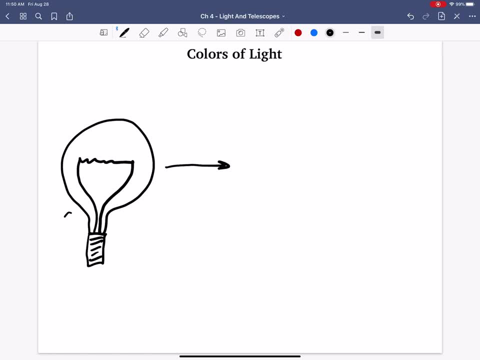 yellow. But what's really going on is that when that light bulb glows right, we see all colors of the visible part of the spectrum. We don't necessarily notice all colors, but we see them. They're in there And we call that light white light because it's comprised. 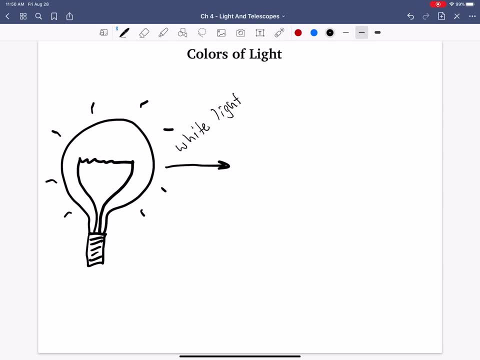 of all the different what we know as colors. And so if we were to somehow break up that white light into the constituent colors, say if we put a prism right in front of the white light, like on Pink Floyd's Dark Side of the Moon? if you don't know what that is, stop this video right now. 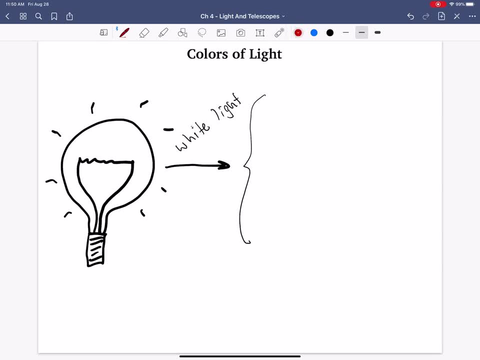 and go watch that, then come back. If we were to somehow break up the white light into the colors, we would see: well, let's go thick. We'd see red light, right, And then next we'd see orange light, Next we'd see yellow light, even though you can barely see it on this. 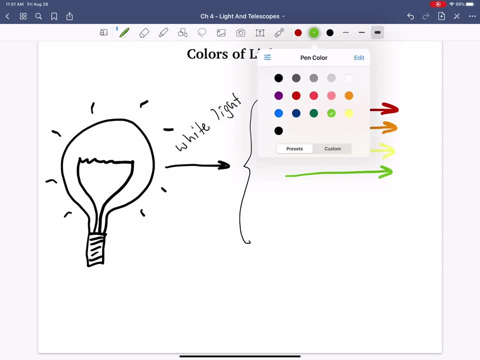 After yellow we'd see green, After green we'd see blue, And after blue we'd see indigo or violet, which is just basically purple, right, These are all colors of light, right? What we've come to define as a color- red, orange, yellow, green, blue or violet. okay, But really they're just 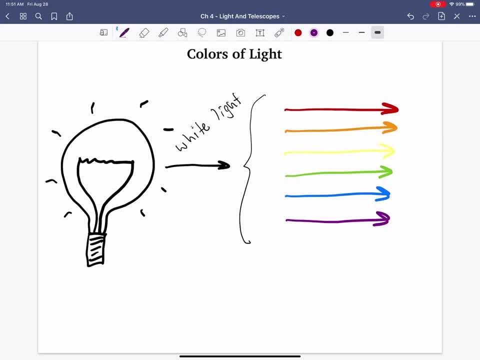 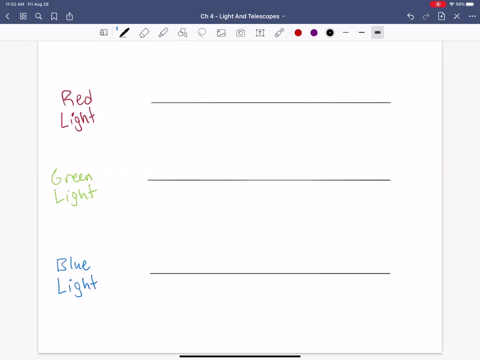 very specific forms of light And I've drawn them as arrows, but let's take a little closer look as to what they actually are. right, Each of these arrows are actually waves. So on this slide here, what I'm going to draw is crudely draw. 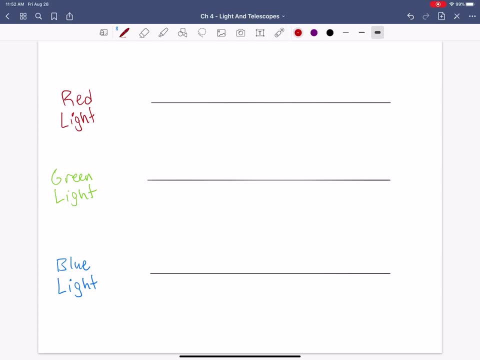 is, or are, examples of various colors of light: right, Red, green and blue. I have the low energy, medium energy and high energy, respectively from top to bottom. okay, So here's an example of a red light wave. Let's go that one. I'm going to draw one wavelength. 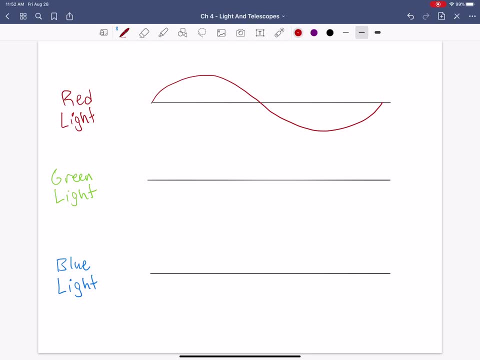 in this space. okay, That's one wavelength of a low energy red light. So let's put low energy, okay, Next with green in the middle. green has slightly higher energy, then red. And remembering back to the relationship between energy frequency, 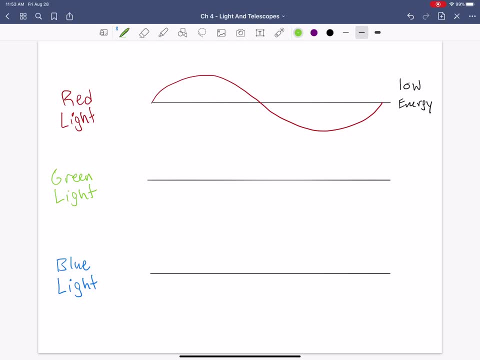 and wavelength right from your textbook. green has higher energy because it has a shorter wavelength, So I'm going to draw that shorter wavelength as one half of reds, okay, So now green has a wavelength of- well, let me just go ahead and draw it Above here. red had 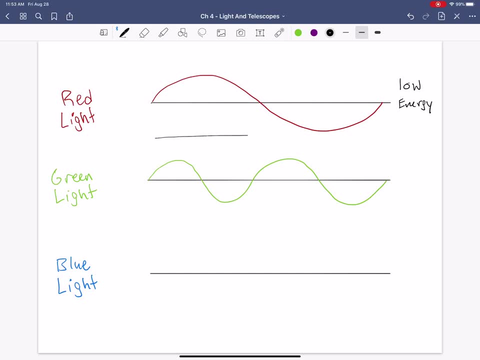 this as the wavelength. okay. Now green has this distance as its wavelength. okay, It's one half of what red's wavelength is, because green has slightly higher energy, what I'll write as medium energy. And so now, comparing green and red to blue, let's see what blue has right. 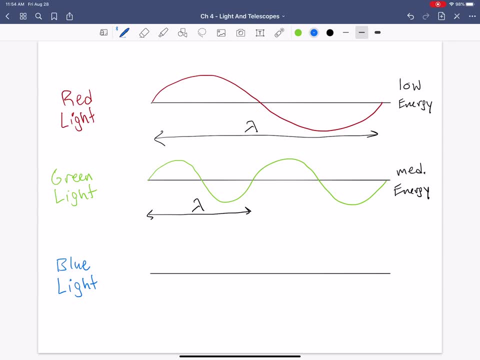 Blue has a wavelength of- well, let me just go ahead and draw it. Blue has even smaller wavelengths, and so it has to have a higher energy. So I'm going to try and manifest it as like this: One, two, three, four. Close enough, right? So notice now. 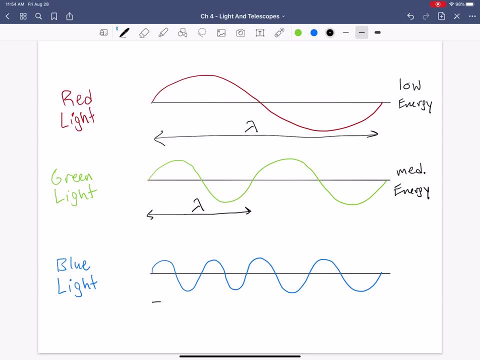 the wavelength for blue is only this far right. That distance is half of the distance of green Green's wavelength right Up there, And the blue wavelength is only one quarter the wavelength for red. Oh crap, It's only one quarter the wavelength of red. So what's happened overall is that. 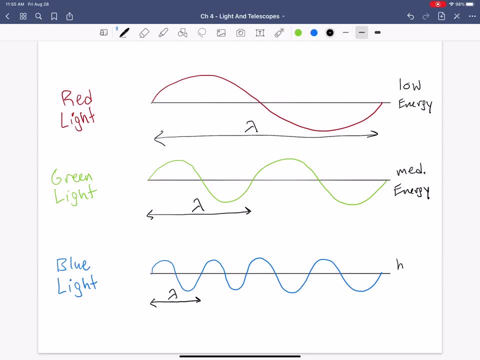 as we've decreased the wavelength, right, the energy has increased. What about the frequency? What do you think the frequency has done? What's the relationship there? All right, Remember, the relationship is that energy is related to or proportional to one over the wavelength, which means that as the wavelength value gets bigger and bigger, 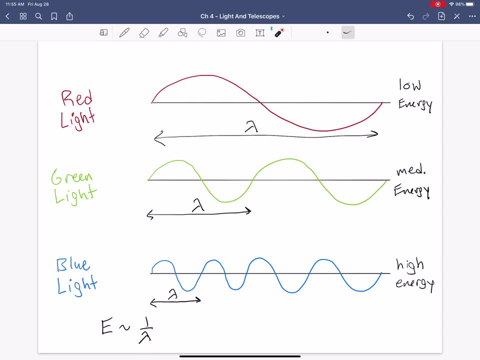 this fraction overall gets smaller and smaller. Thus, the energy gets smaller and smaller, And that's exactly what's happening as you go, say, upwards on this page. If you go down, the wavelength is getting smaller and smaller, And so this fraction overall is getting bigger and bigger and we see a higher value for energy.